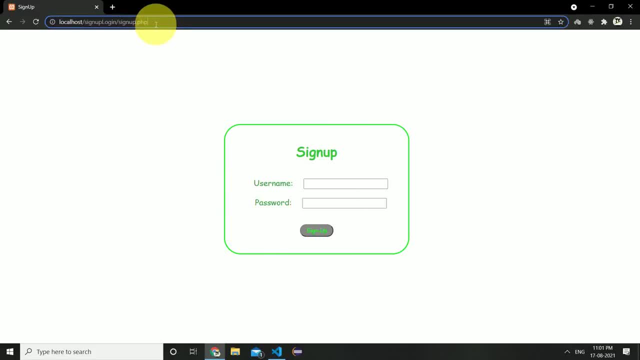 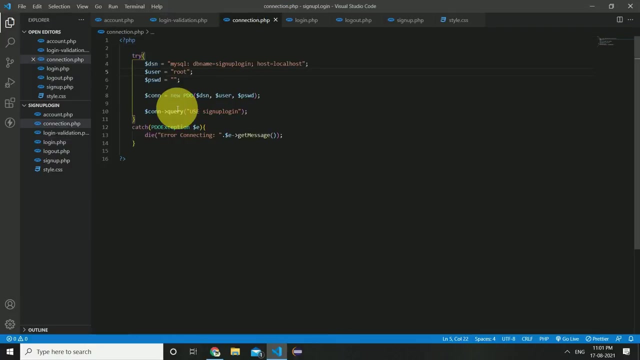 Hey guys, in this video we are gonna see how to upload your PHP MySQL website to internet for free. Yes, it's possible. you can host your website with database for free. This is a sample website created using HTML, CSS, PHP and MySQL. 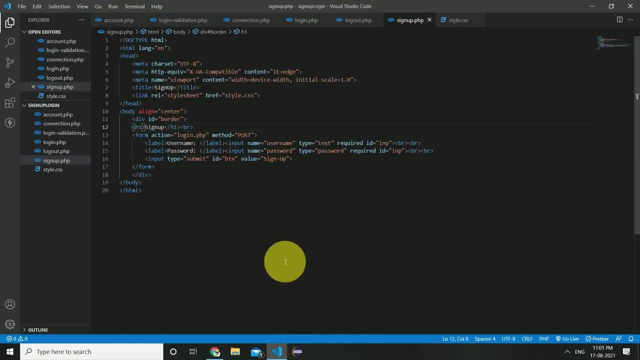 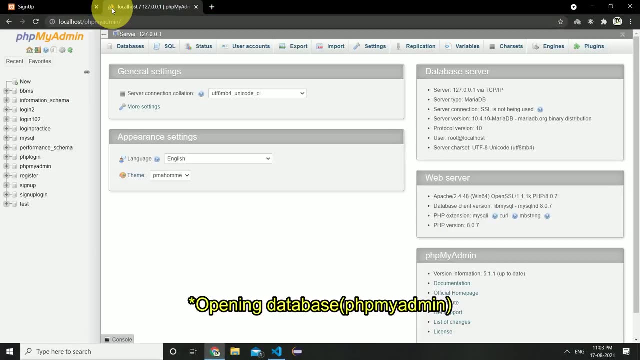 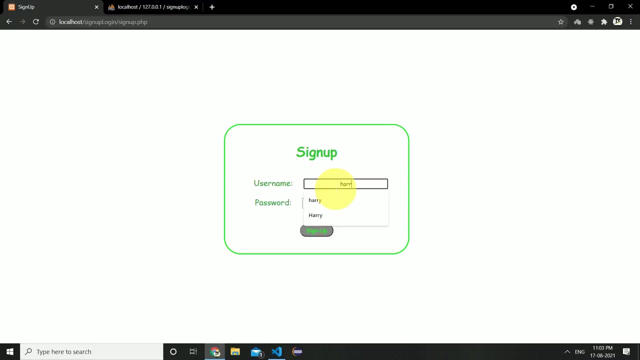 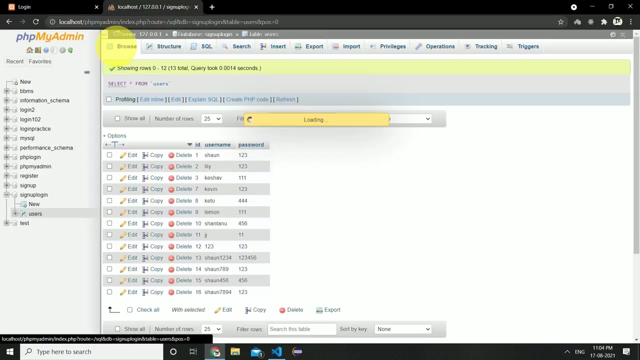 I'm gonna host this website live for free. while demonstrating you all, Let me show you this website. first, Let's sign in. harry123, and password123. Account created successfully. Now let's check the database. Yeah, the username harry123 and password123 is stored inside the database. 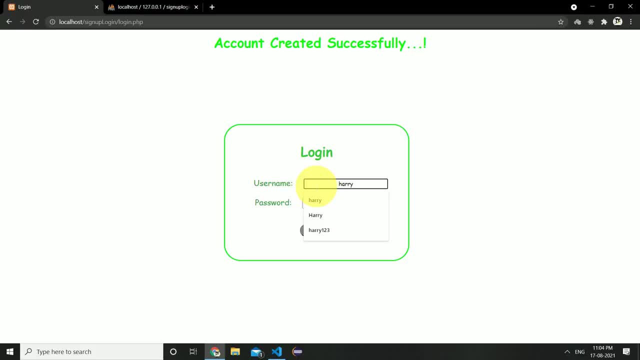 Now let's see how to put this in the database. Let's open this site on internet for free so that we could be able to share it across the globe. And guess what? you will find link to this website below in the description box. 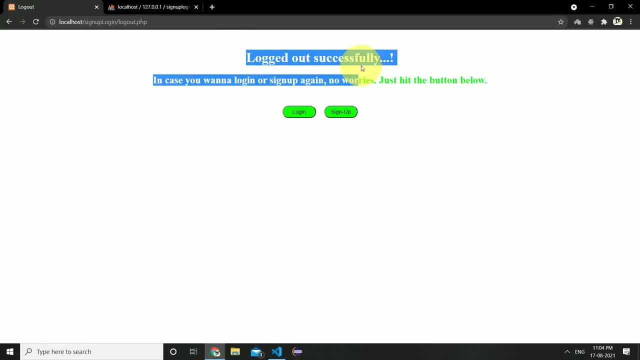 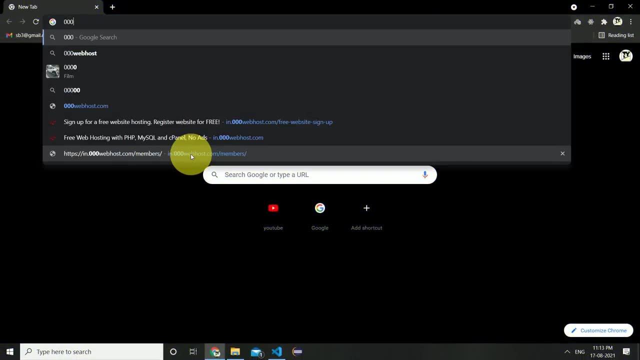 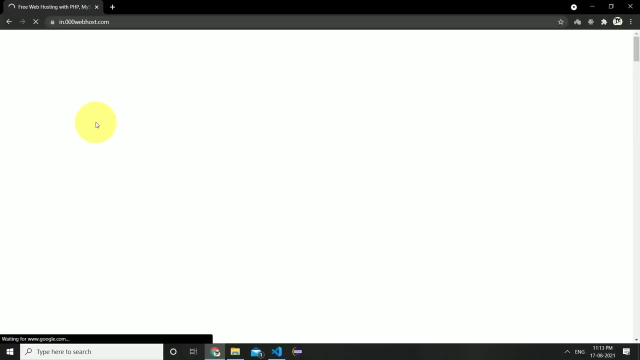 as a proof that it's live and hosted successfully. So, without any further ado, let's get started. Firstly, open any browser and search for 000webhost. You can also find link to this website in the description box below. Once you open this website, click on get started. 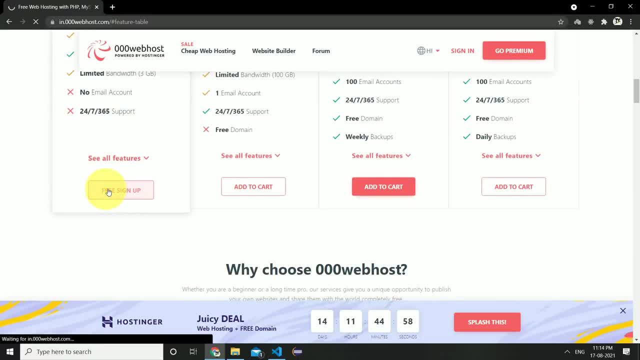 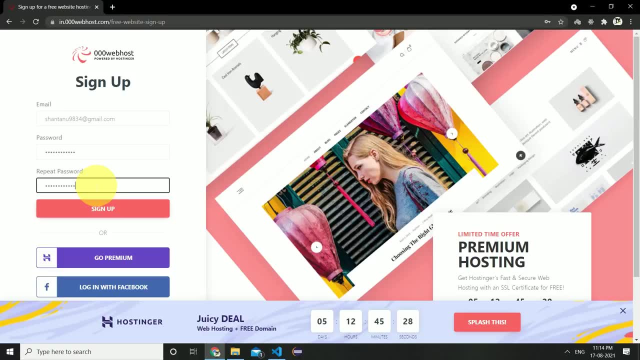 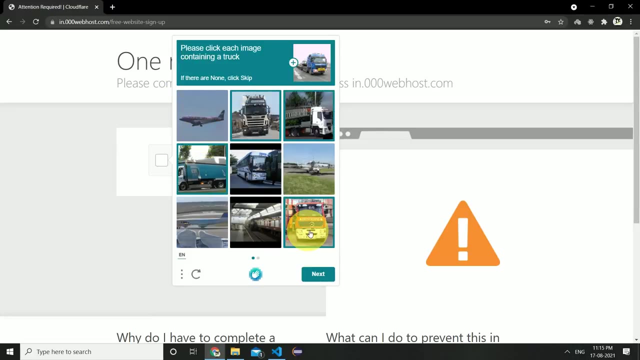 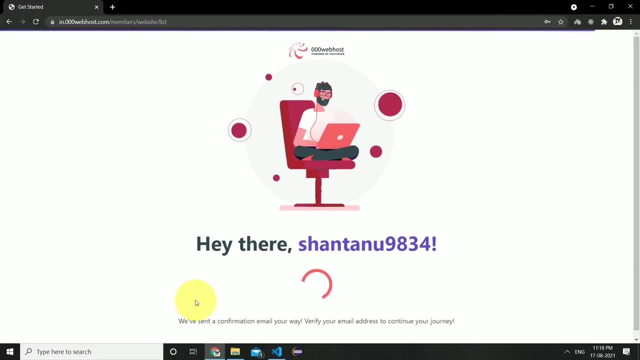 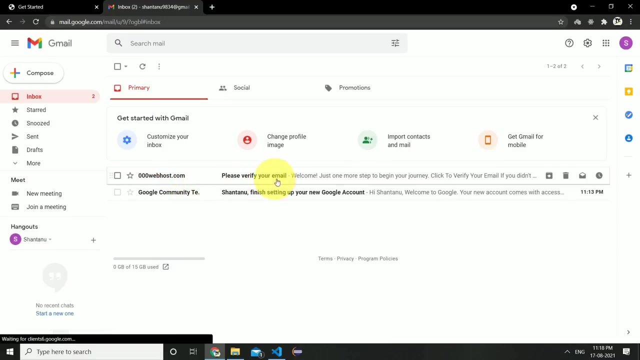 Then select the free sign up option Here, enter your valid email address and password and press the sign up button. Then complete the security check And you will be redirected to this page where it says to verify your email address. So open your email in a new tab and click on the verification link over here. 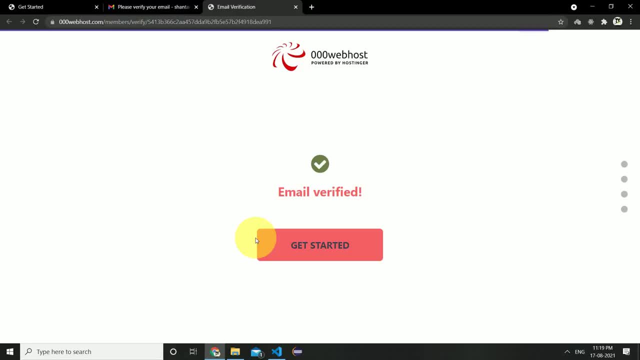 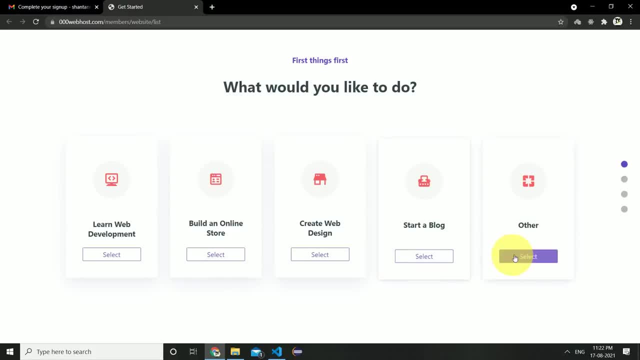 And you will be redirected to this page. And you will be redirected to this page. And you will be redirected to this page. Here, select the other option And this page will appear. Here. you have to enter your website's name. In my case, it's my mini project 2021. 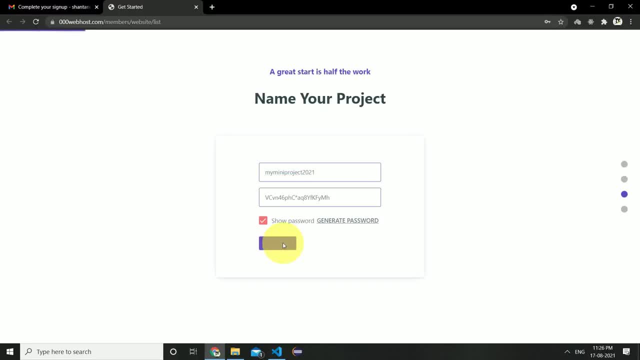 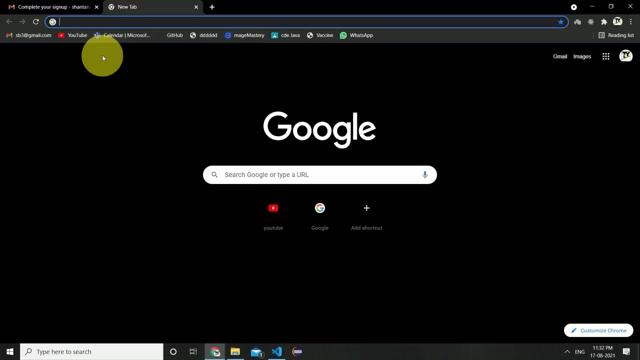 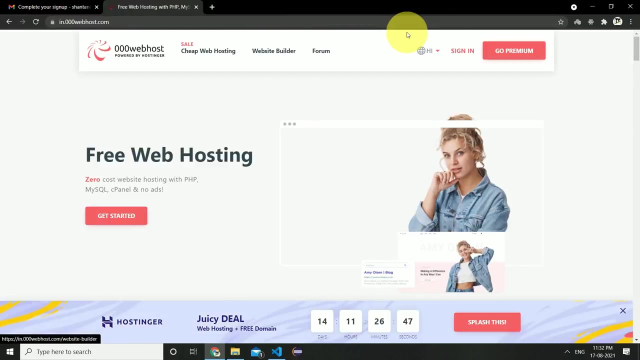 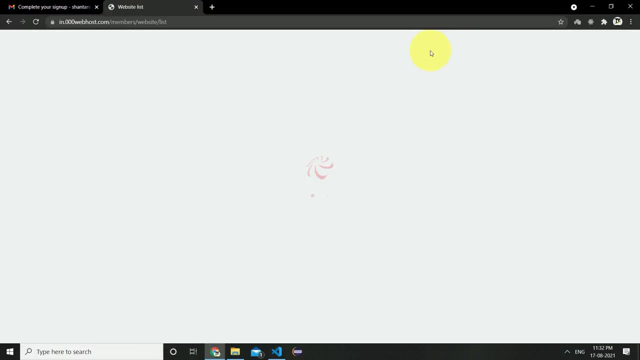 And leave everything else as it is and click on submit button. That's it. now close everything and once again open the same website, 000webhost, And this time click on sign in. Here you will find the website that you just created. 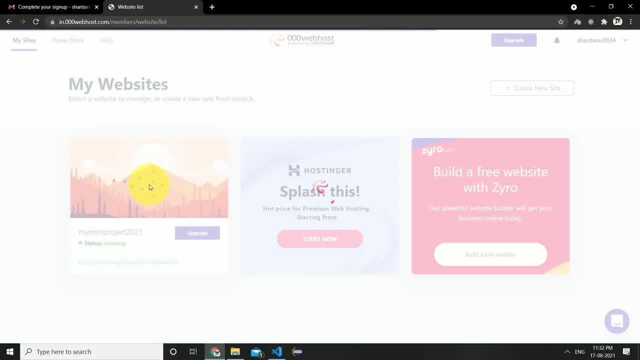 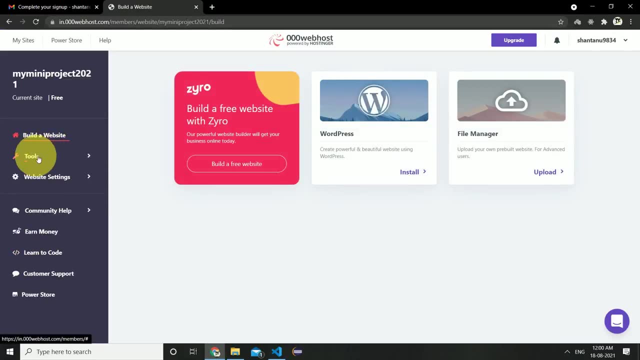 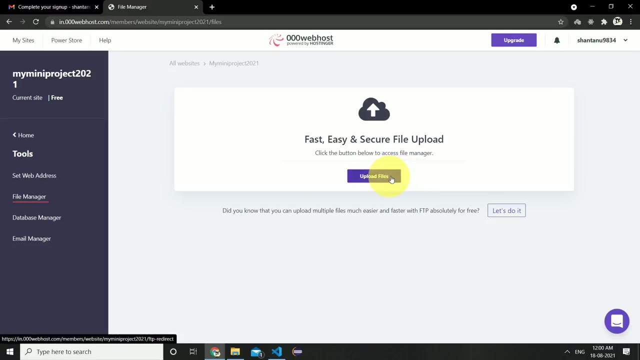 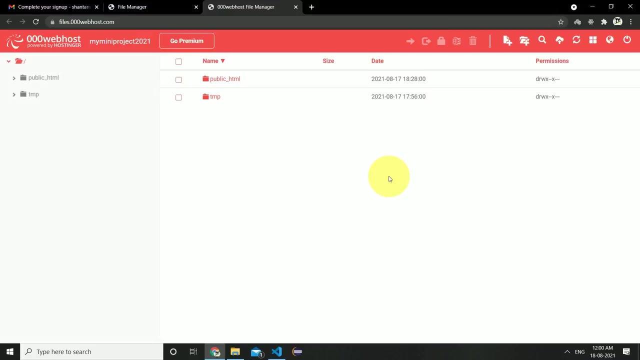 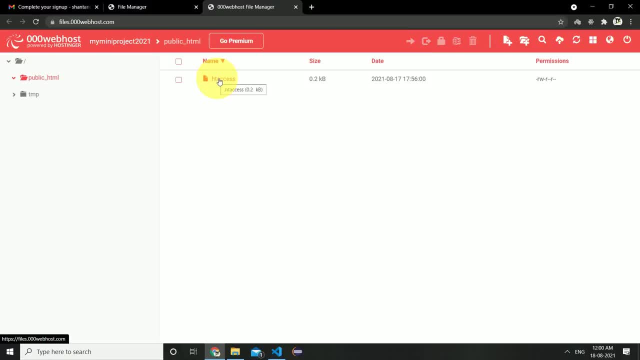 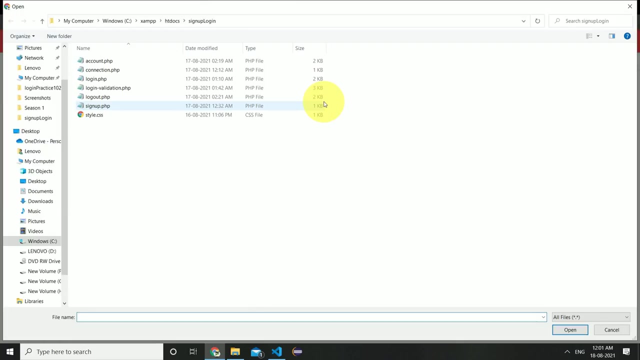 Here. double click on public html folder After double competing, click on upload. then click on upload. Then click on the upload icon on the top right corner. Now click on select files. Now browse and select all the files that are needed for this project. 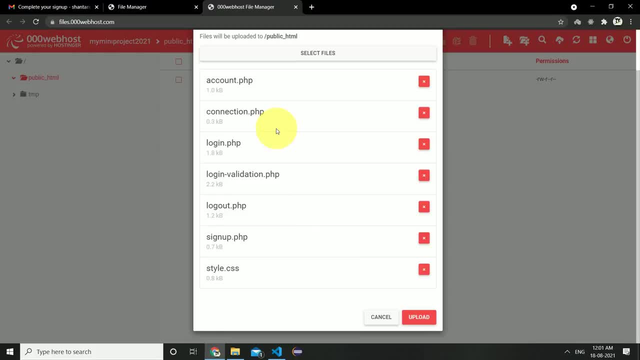 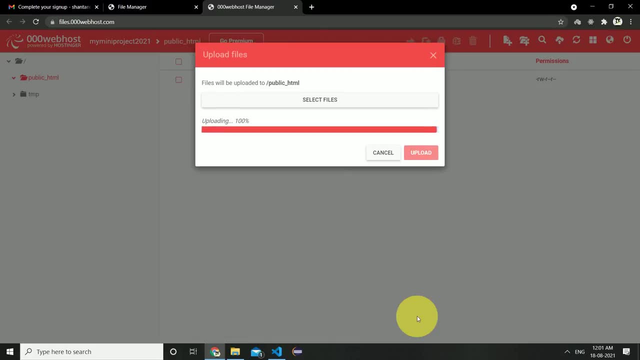 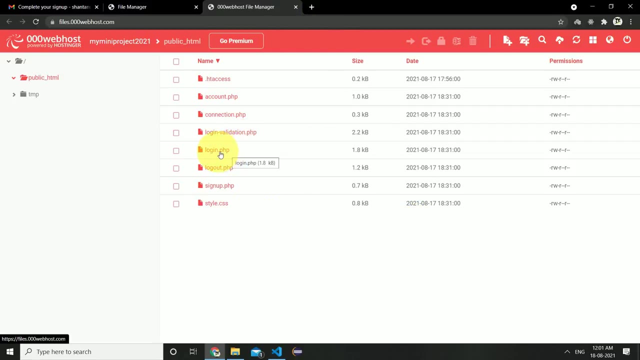 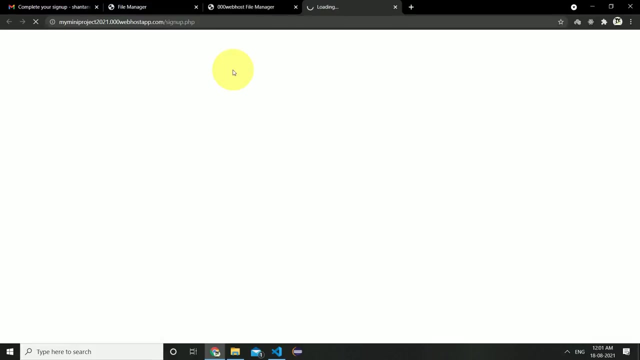 And click on open, Then click on upload. After uploading all the files, right click on your home file or index file. in my case it's signupphp, so I'll right click on signupphp and click on view Here. our website is hosted live, but we haven't connected our database yet, so it'll show. 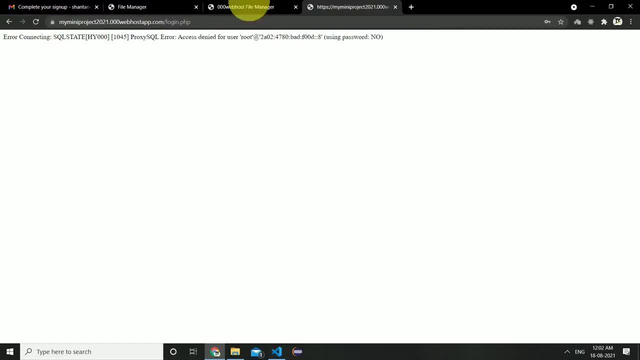 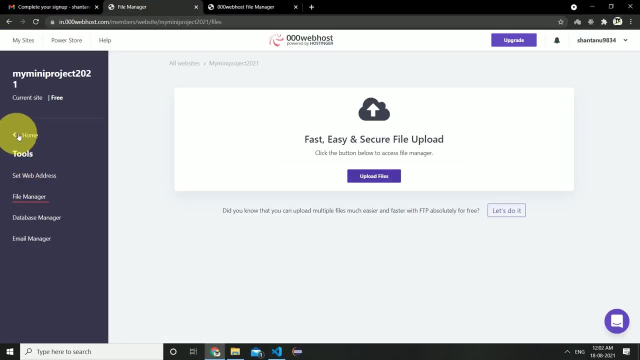 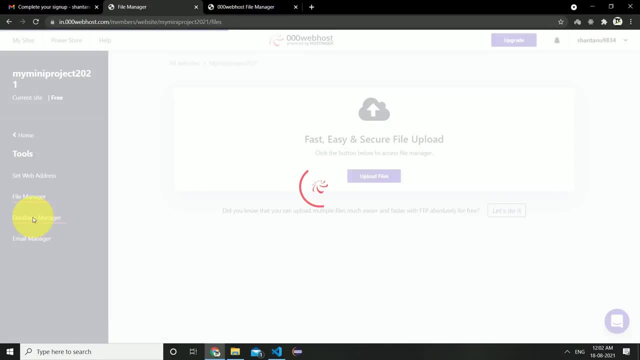 error. Now let's connect this website to database. So, in order to connect database, come back to your website's dashboard Now click on database manager over here. Once you click on database manager, this page will appear Here. click on new database. 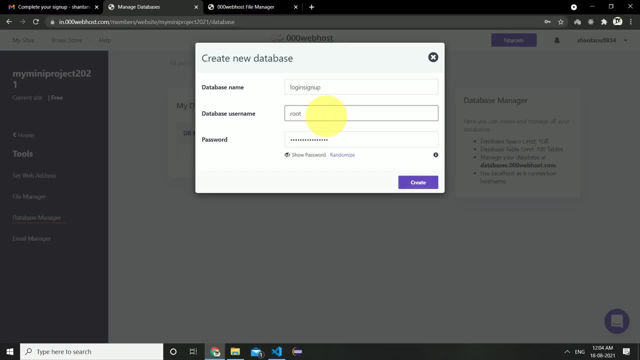 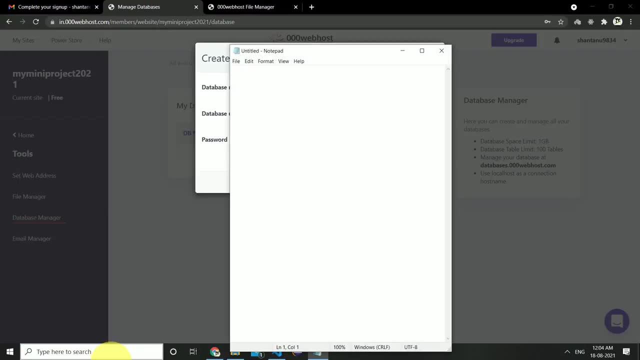 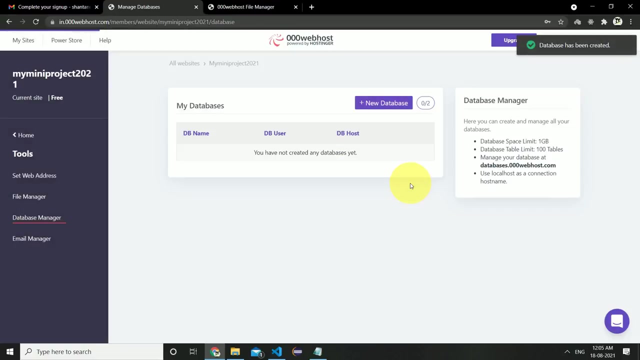 Now enter whatever database name and username you want And click on show password. Then open notepad And copy the password and paste it inside the notepad. Now click on create Here. it'll take some time to create database. Once the database is created. 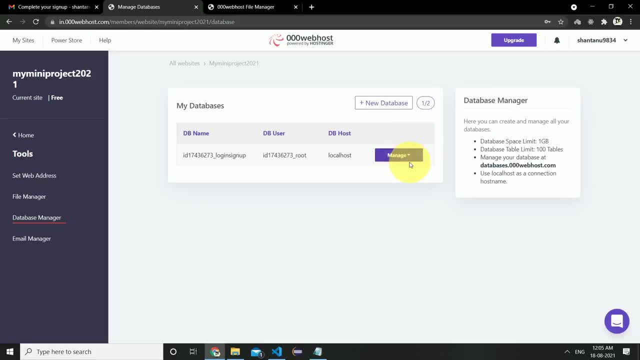 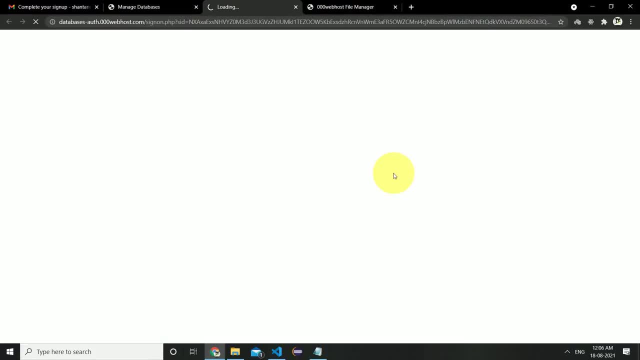 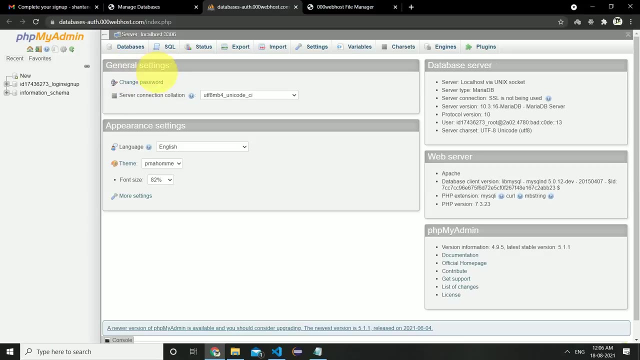 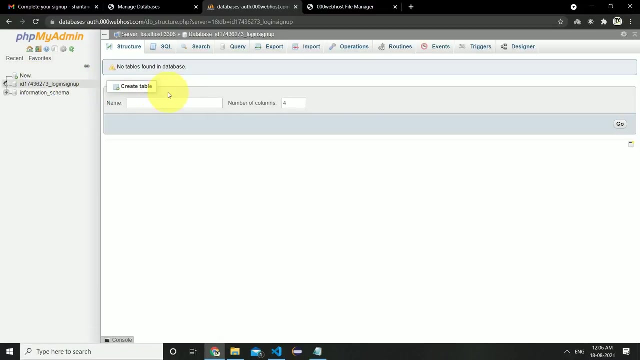 Go to the homepage And then click on create created, click on Manage and select phpMyAdmin. Here we'll click on our database. Now we have to create the same table with same names as we created earlier on our phpMyAdmin. 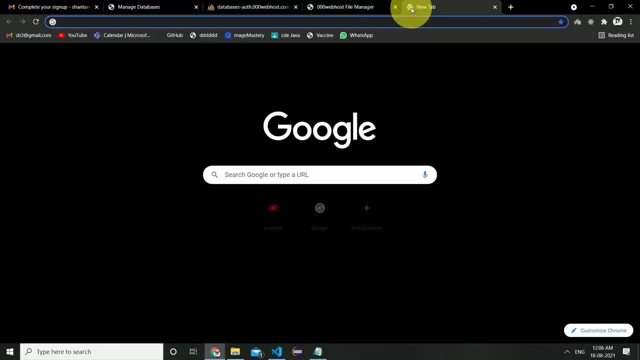 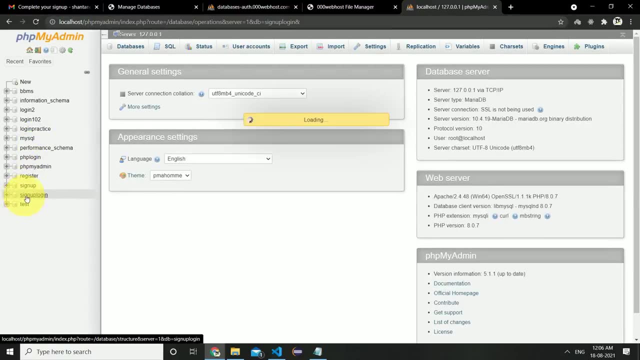 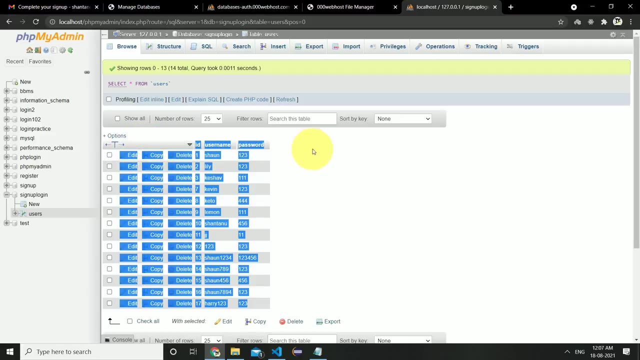 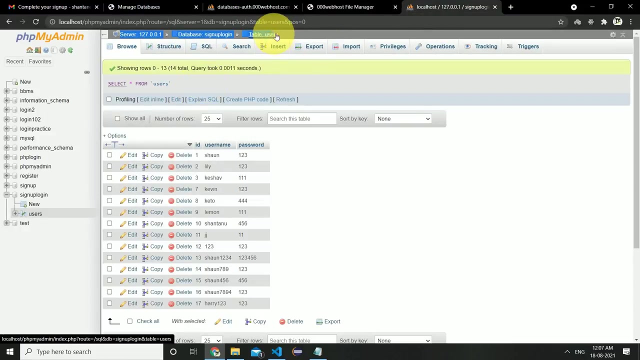 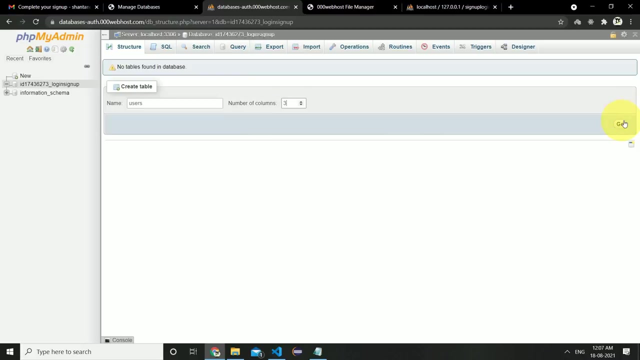 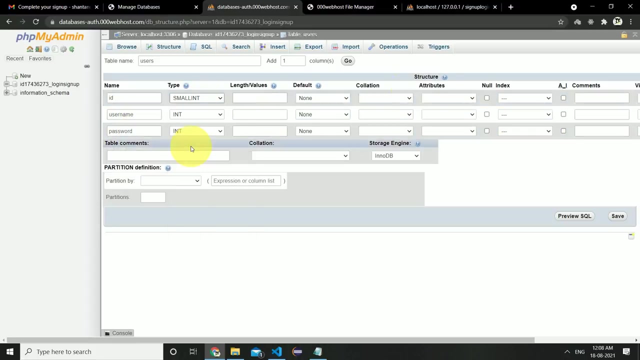 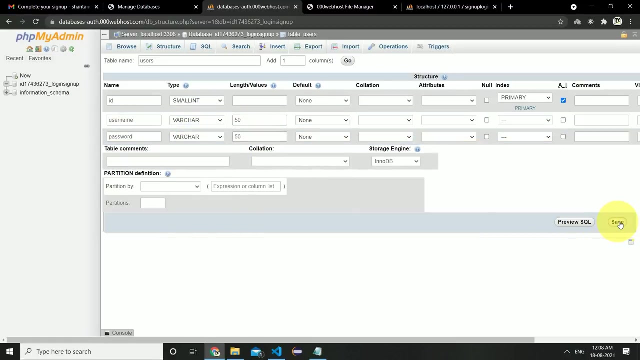 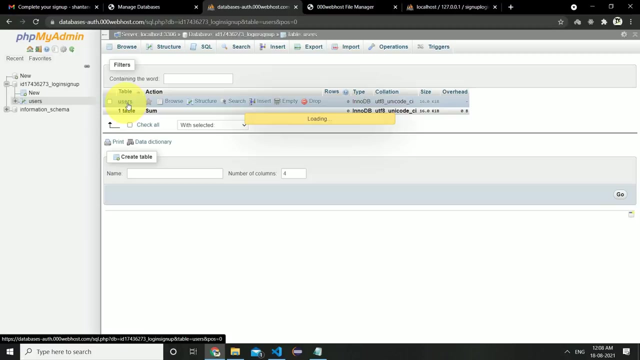 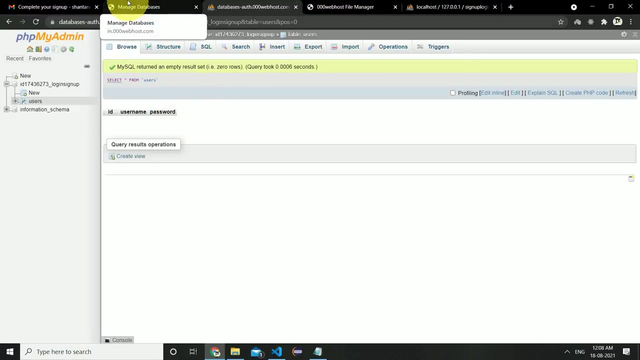 from XAMPP. This is our user's table from XAMPP phpMyAdmin, and now I will create exact same table inside website's phpMyAdmin. Ok, so we have created our user's table successfully. Similarly, you have to create your table.